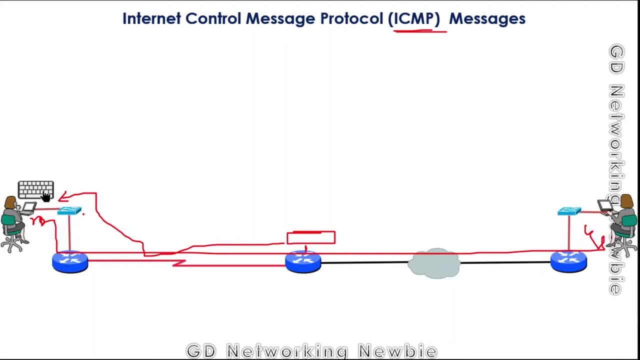 these are the purposes of this ICMP protocol: to check the connectivity and reachability of the nodes. so these are two ICMP protocol and for that ICMP itself uses some messages and we are going to discuss those messages in this video. so this is a protocol. ICMP is a protocol that is used for error reporting. 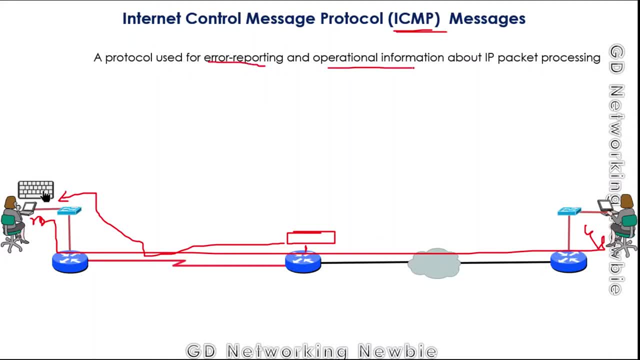 and some some signing, some operational information about IP packet processing and this is actually a network layer protocol. so it is here some network layer protocol and this is ICMP. then this ICMP itself, so ICMP packet itself is encapsulated in an IP packet, and then we have ICMP header and then we have the rest of the things there. it means this is: 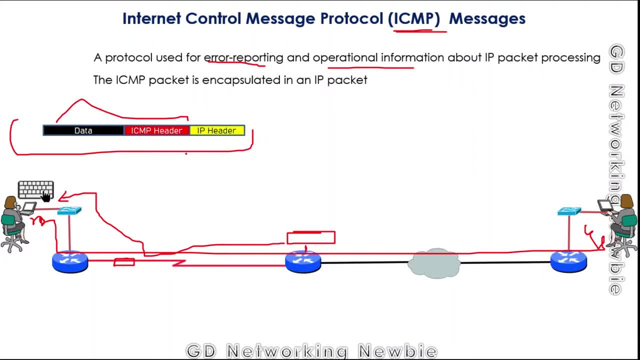 some IP and we have encapsulated this thing, this ICMP, within that. so this is the big container, and then this is something small being put back into. this is on this ICMP씡 layer arrestor. so this something is very small. we put that into this container. now, this is the same thing where our 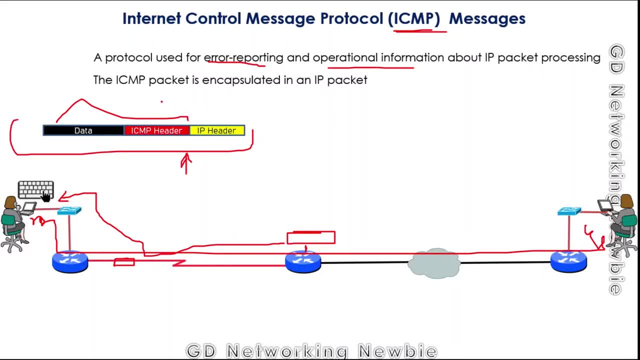 that content, i might say so that's encapsulation about icmp packet and let me remove this now in this icmp header, what we have. so if we saw that this icmp can generate some messages and those messages can be sent to the source, but how this is done by icmp protocol and for that we need to look. 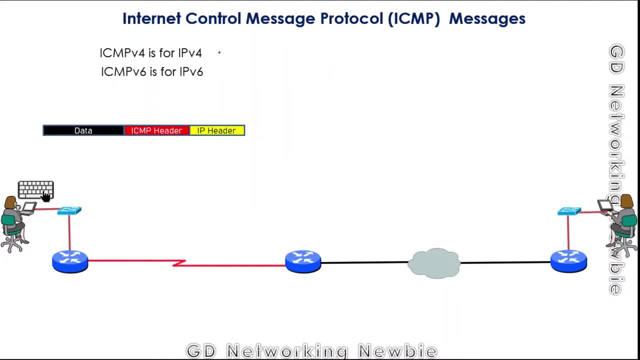 into this icmp header. but before that let me mention that there are two versions of icmp. one is icmp version 4, that is used for i in ipv4, and then we also have icmp v6. that is version 6 and that is for ipv6, and in both of these protocols and both of these versions we have different. 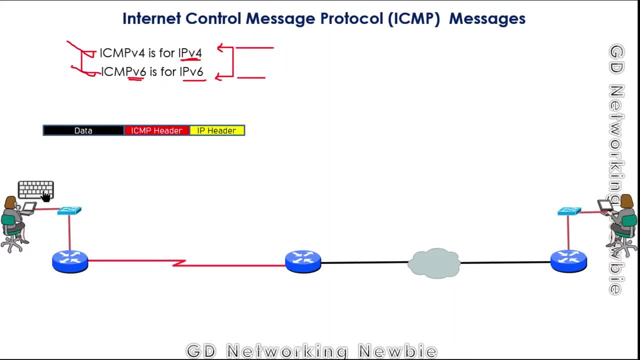 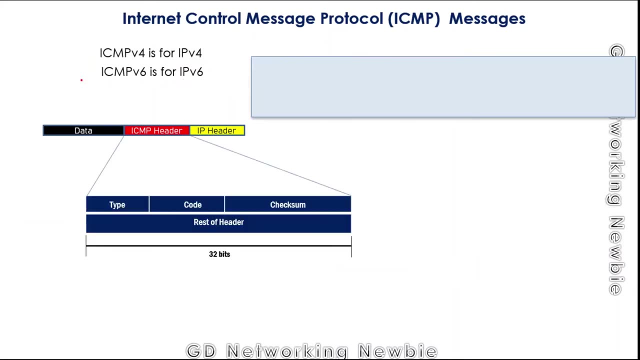 messages, but there are some of the messages which are common to them. it means those messages are common for this as well as this, so we'll be discussing some of the common messages in this video. let's go and see what is in this icmp header which is used and which is going. 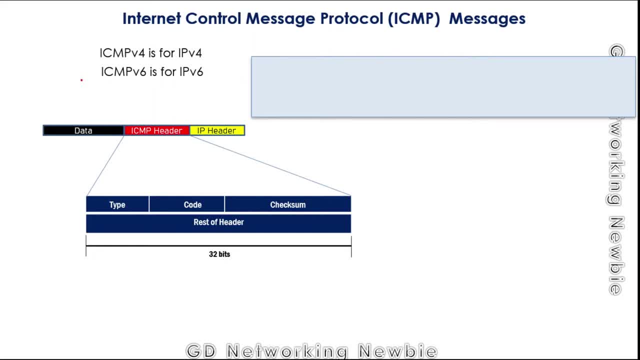 to send some messages to the host and which is actually used for diagnostic purpose. so for that we let's explore this icmp header. so before that, i want to emphasize that this icmp header actually will be different from one one icmp type to other icmp types. it means there are different. 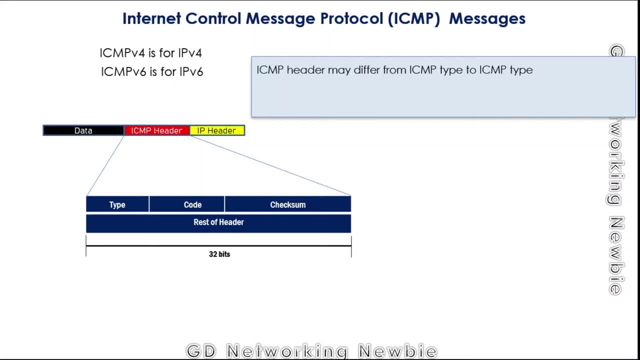 types of icmp and for every type or icmp type message we will have a different header there. so this is a general header and all icmp packets have an eight byte header and variable size data section. so header length is eight byte of this icmp header and out of those 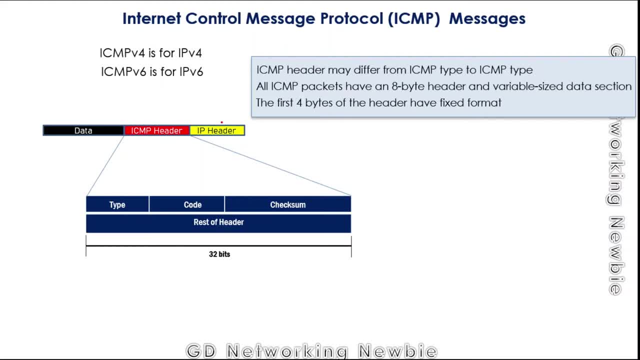 eight bytes. the first four bytes of the header have fixed format, so the first four bytes. so here this is actually four bytes. this is 32 bits. you can see this is eight bits, eight bits and 16 bits. so the first four bytes have fixed format and i'm going to present that fixed format for. 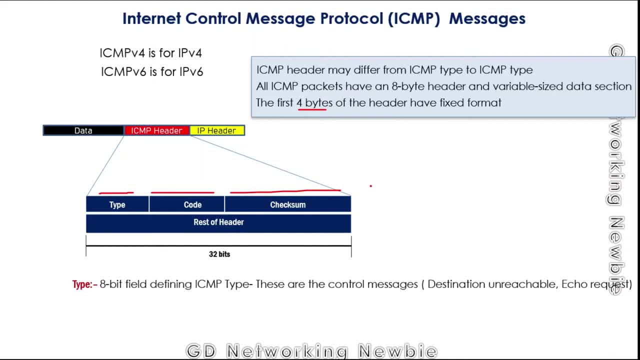 this icmp header here. so in this, in this icmp header, the first field, which is this, which is the type field, that is actually eight bit field, and this field actually defines the icmp type. so icmp type means there are different control messages, like we have destination unreachable, maybe we have the echo request: equal reply. so these are the types of 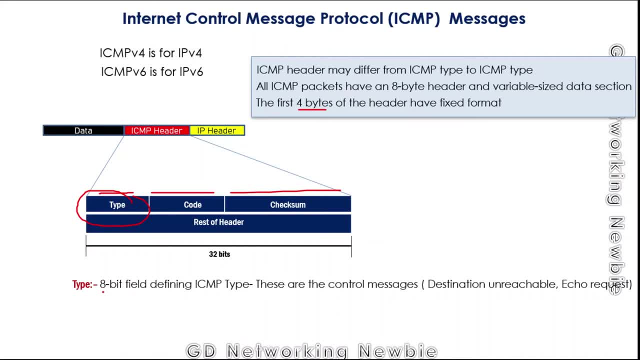 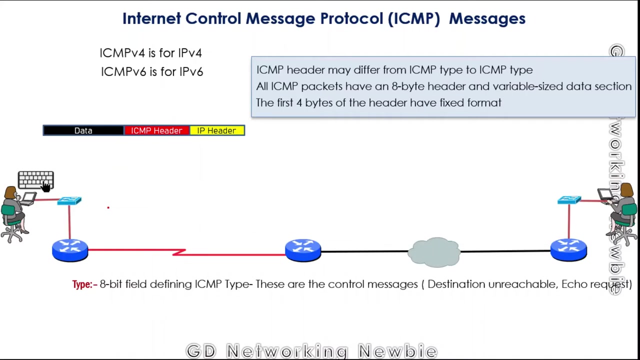 messages and what type of messages are. what type of message is being carried at particular time that is actually indicated by this type message. that can be maybe just destination unreachable. that message can be echo request, so that is actually identified by this field, that is type field. so for example, here we have, we have a network, so this user is sending some message. 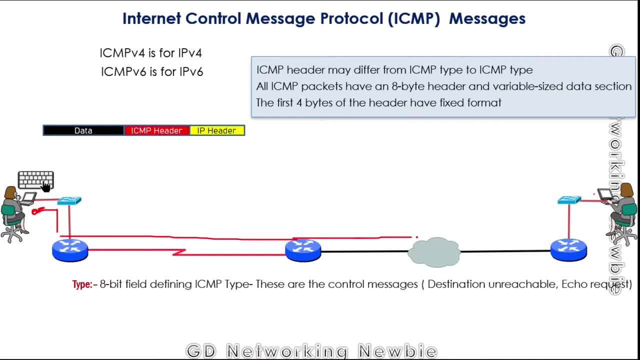 to, maybe, this destination and when this message or when this data or when this packet actually arrives at this router- and due to some reason, if this, this router is not able to send that, that packet to the actual destination, then the router can generate a destination unreachable message- router cannot deliver it to the actual destination- and then, in that case, a router. 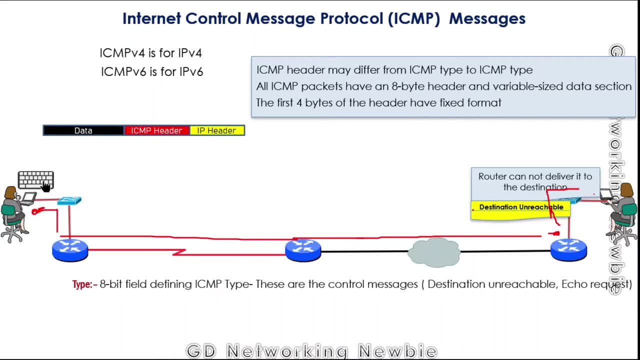 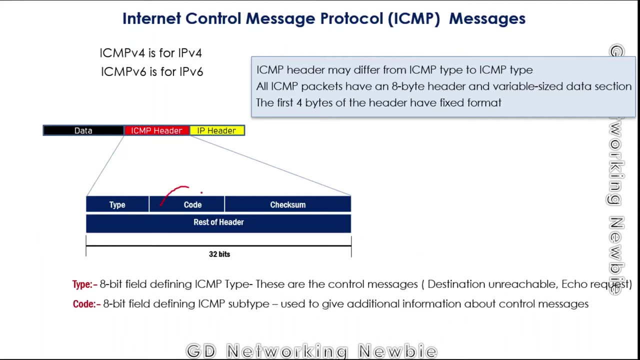 can generate a destination unreachable message and then this message will be sent back to the host to inform the host that your message was not successful. after type field, we have a second field, that is code field. here, and code field is again an 8-bit field, and that defines are: that is actually the subtype of. 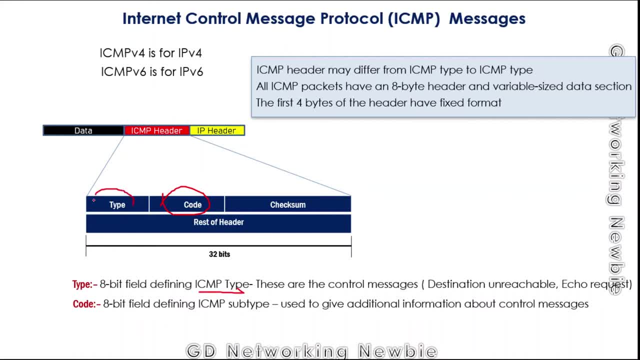 that icmp type. we have icmp type broad category and within that further specification about that type is given in this code field and that is giving us the additional information about this message which is selected in this type field. for instance, we have functions. we say that we have. 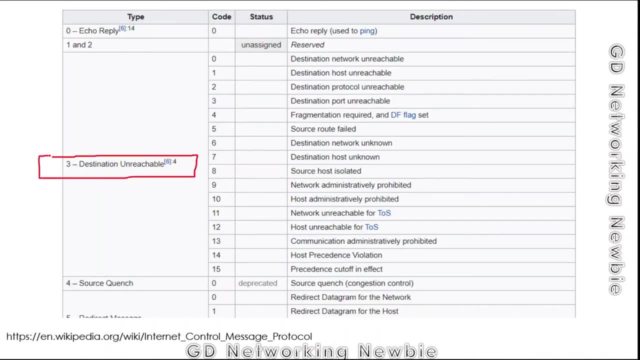 this field, here in the type field. so in this case, in this type field, we saw that we have this code. that is three, that is, that the type type of message is destination unreachable, but further information about that destination unreachable, that why this, this occurred. so for that we have codes and in this code, for example, in this destination unreachable, we can see: 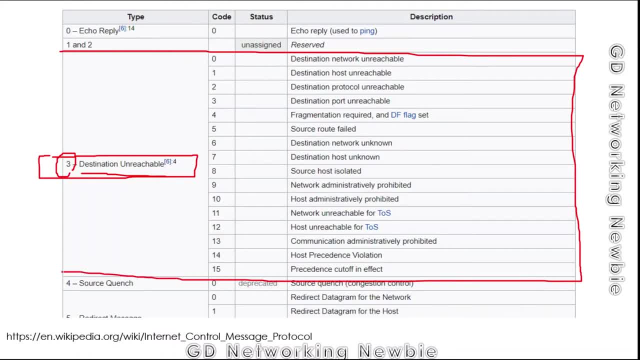 that we can have different reasons for this destination unreachable. what is the specific reason for this destination unreachable? that is basically indicated by the code field. and here you see, in this code field we have zero, it means destination network unreachable. if scope is one, it means destination host unreachable. 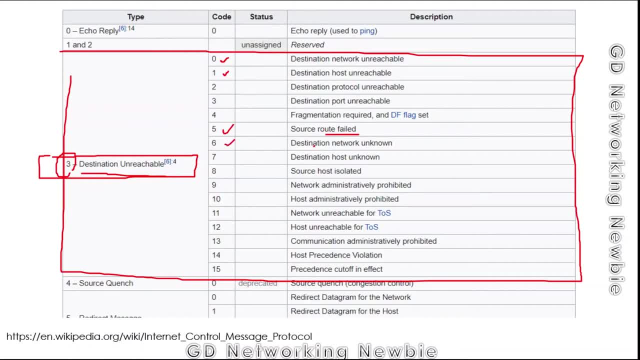 if this is five, source route failed. for example six: destination network unknown. destination host: unknown. we can see within this simple type or within this single type or icmp type of message, there are different reasons and those reasons are given in this code field. so this actually code field is gives us the further. 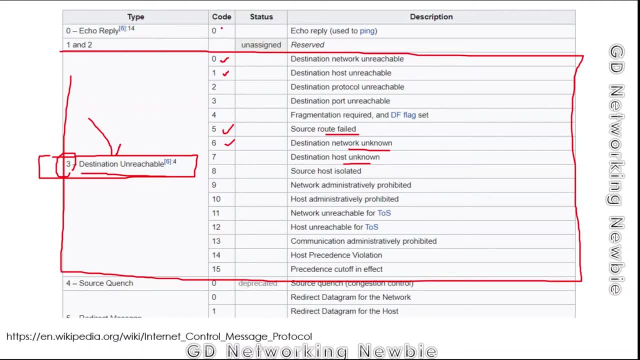 details at what happens. so in some of the type of messages we can have only single code and some of the icmp types of message can have multiple codes to give us the additional detail. so these are fossil echo requests. we have this destination unreachable, we have source quench and i have taken this information. 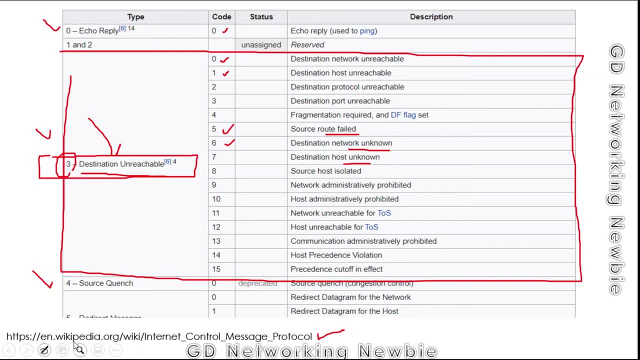 from this wikipedia and have given this link. you can go to this link and read about all those messages, icmp messages, which are there. so i'm not going and not be going through all those messages, but i'll be discussing only few of them, but this is a really useful resource. on. 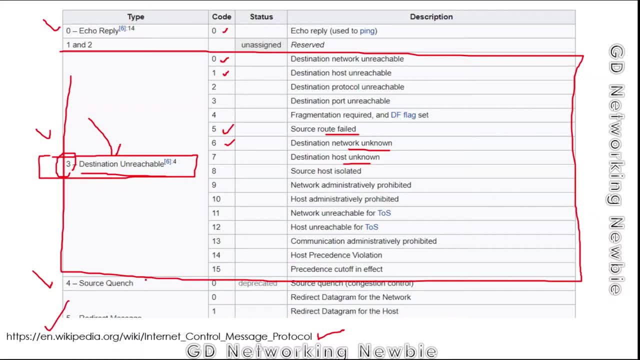 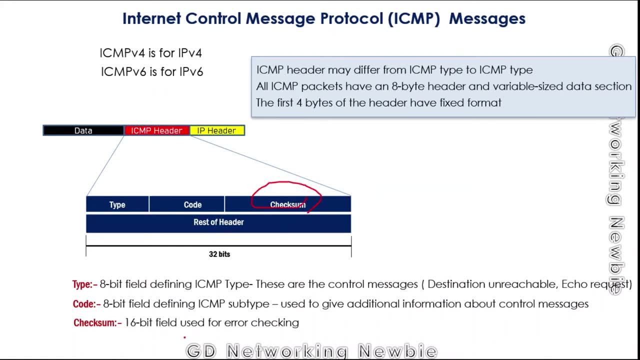 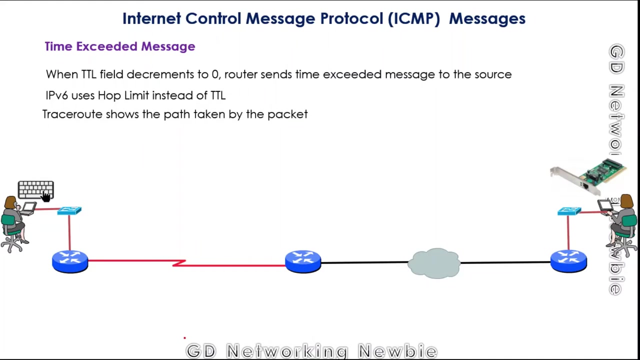 the wikipedia. you're recommended to see this one if you're interested. and now the last field is the checksum field. the checksum field is a 16-bit field that is used for error checking, not correction, but only the errors will be checked and then some of the icmp messages we we can see here. we can go to that wikipedia as well. 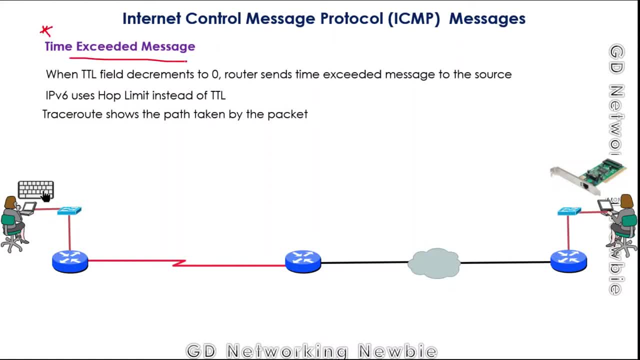 so one of those icmp messages is time exceeded messages. so time exceeded messages is used when this ttl field is decremented to zero. so what is ctr field? so that is time to live field and if you remember, then in ip header we have a field that is time to live field. 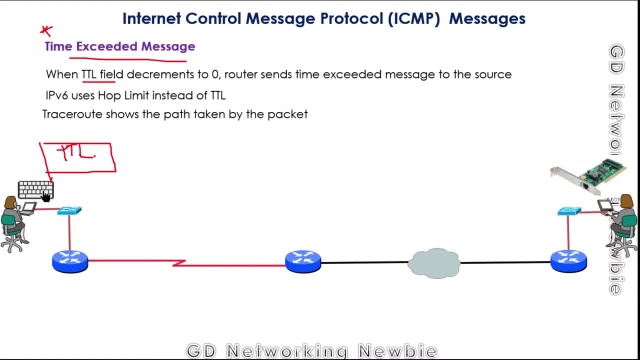 and that time to live field is used to to specify a lifetime of the packet. okay, so that is actually the hop count of this uh of the packet. so, for example, if the, if the ttl field is two, it means they have the packet can only travel from this to this, so means two layer three. 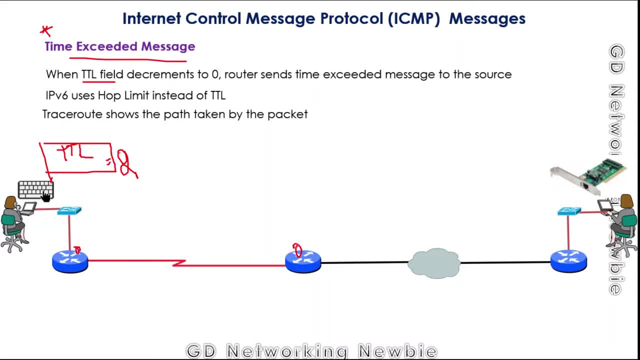 hops can be um can it can be transmitted. by this i mean this packet can can be transmitted to two hops and after that this packet will be discarded. it will not be forward to forwarded further. so when this ttl field expires, as this is decremented to zero, the router sends and time. exceeded message to the source, for example. for example, if we look at the sorry 的 ttl field and if the heinous was increased or if the tiller is decreased to 0, the router sends an action And the time exceeded message to the source. focus on the world, please. I just want to let 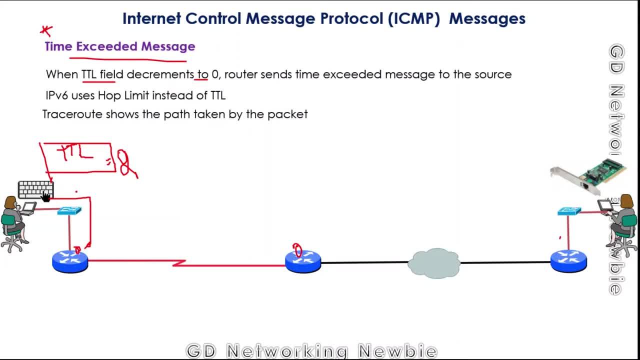 say that this packet arrived here. initially, the time to live field was two, and here this will be decremented by one, so this will be one. and when this received, this is received at this router, this ttl field will be decremented again by one. and now this will be zero. and once this is zero, 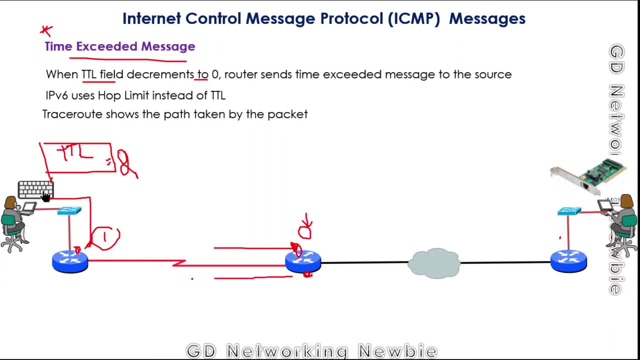 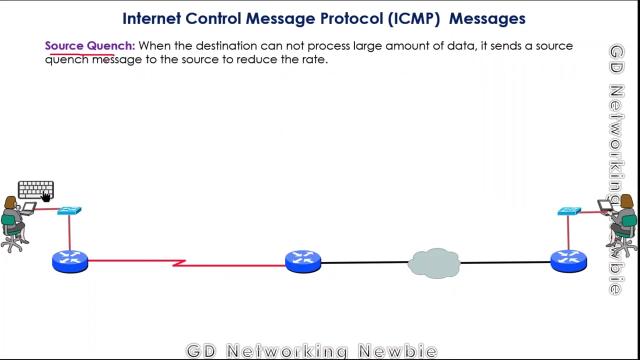 this router is responsible to send back some message to the host that, due to this reason, due to this, some reason of, due to this reason- i mean the time exceeded- message will be sent to the host indicating that, due to this reason, the packet has been discarded. in the same way, though, this is source quench message, so, for example, this source is sending: 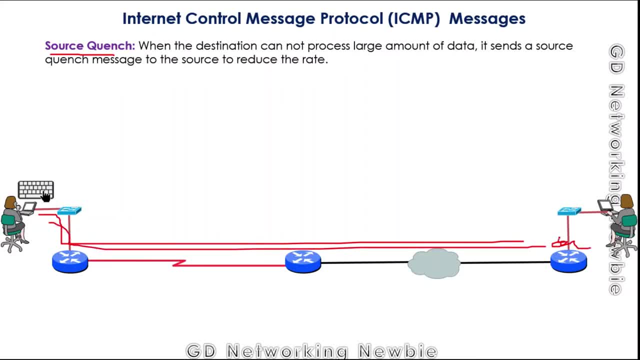 the packets to this destination. so let's say this some point: this destination is not capable to process that a large amount of data, so in that case it can send this source quench message to this to the source: that please reduce the data rate so that i should be able to process it. 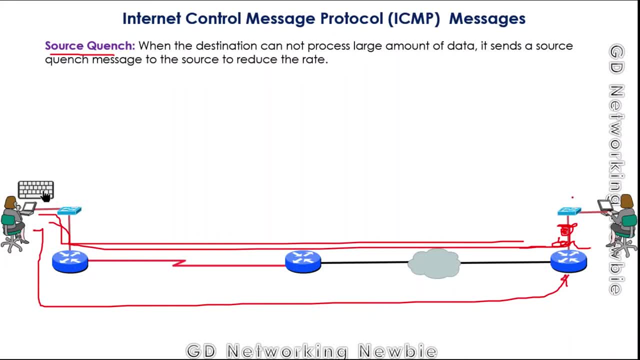 otherwise i will not be able to process it, maybe due to different reasons, maybe the buffer side buffer size is not allowing me, or any other reason, so that's actually deprecated. we have some other ways to achieve the same goal, but the job of this uh type of icmp message is that to intimate the sender to reduce the rate, data rate which 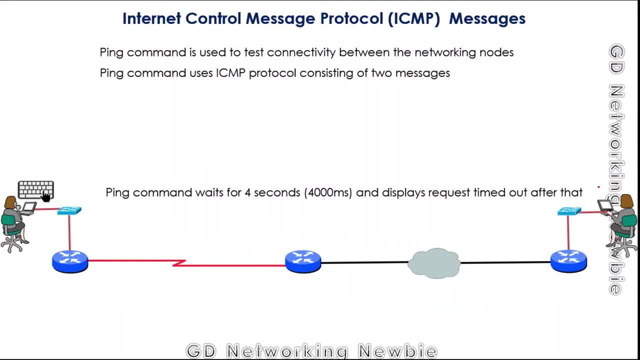 is being sent. in addition to that we have this well-known ping request or the ping command which we used, and in this ping command that's used for checking that connectivity or reachability of the nodes, so that ping command actually uses icmp message. one of them is echo request and second one is echo reply. so i have other. 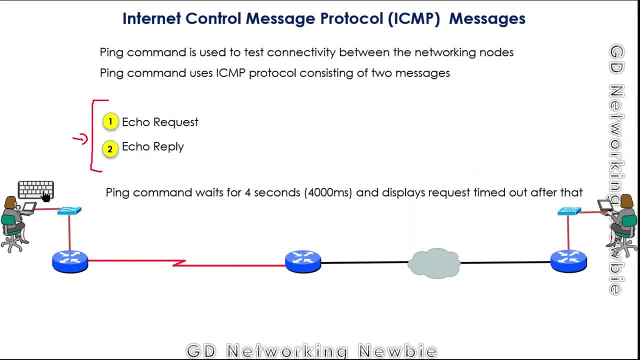 video discussing these things in detail, but here by using ping command. so when we use ping command it means we send some packets to the destination. that is sent in the echo request message and when the destination receives and says that yes, i'm here, then that message is sent back in echo reply to the destination and then in that and in the command prompt. 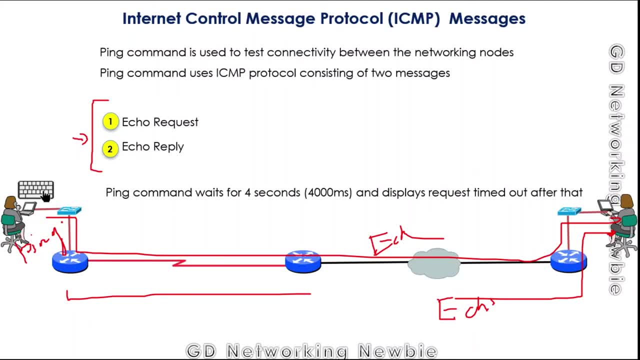 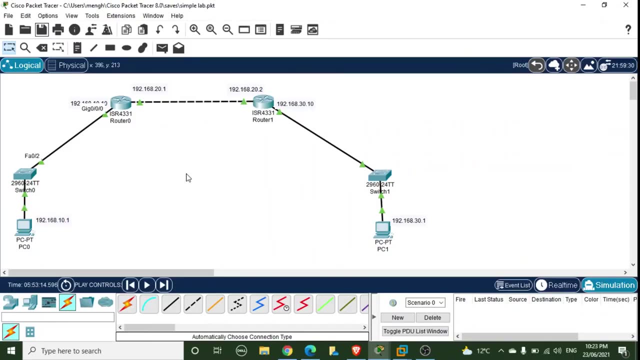 maybe we can see that uh ping was successful. so now these are some of the messages which we discussed, and let's see the same echo request and record reply in packet tracer. now to show you this icmp header fields, i have created a simple lab here. so we have one computer, second computer, two routers and they are connected. 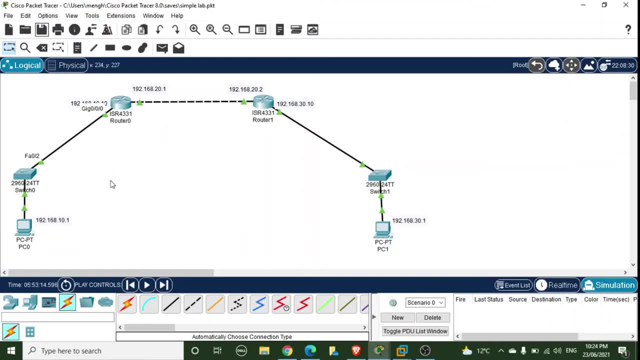 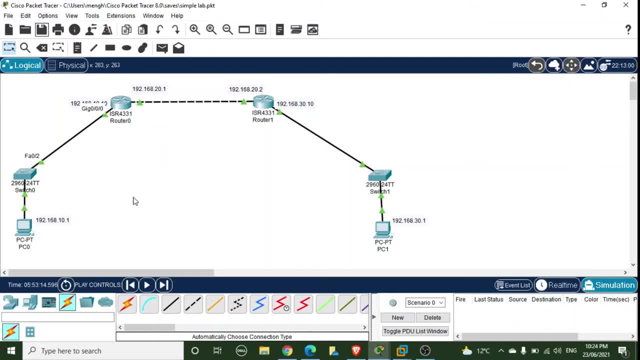 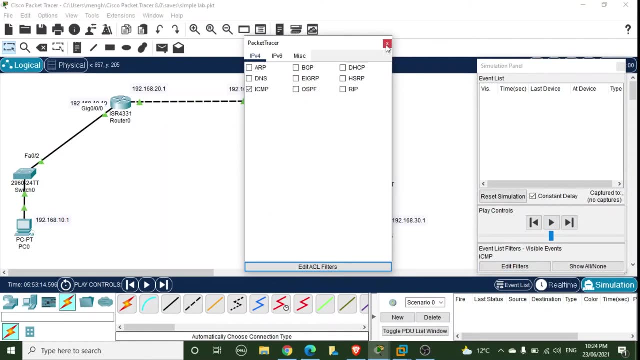 fields look like in this icmp header. so for this i'm going to switch to simulation mode and in this simulation mode we have this window and i'm going to click edit filter and i have just selected icmp protocol and then i'm going to ping, so i'm selecting this simple pdf. 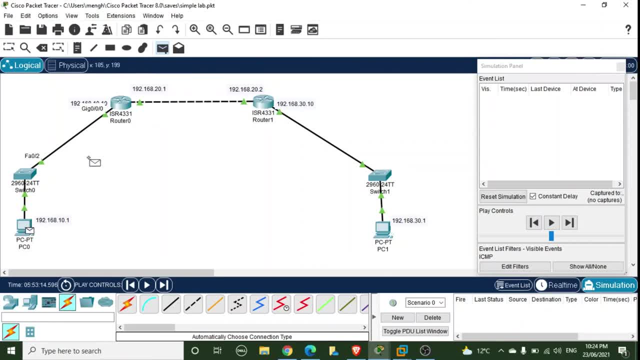 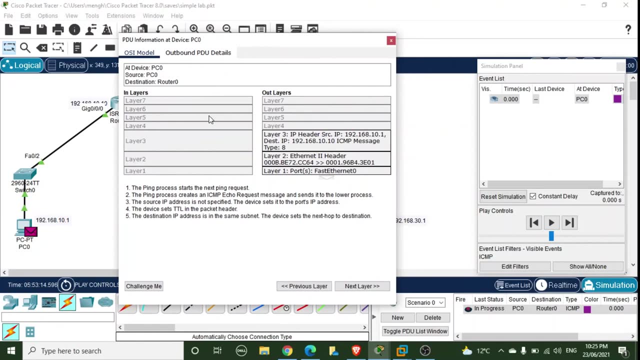 so i'm going to ping from this pt, uh, this pc to this interface or this router and then, once this, this pdu, has been created, we can see what is in its icmp header. so for that, when we click on this outbound pdu, so you can see, here we have ethernet. 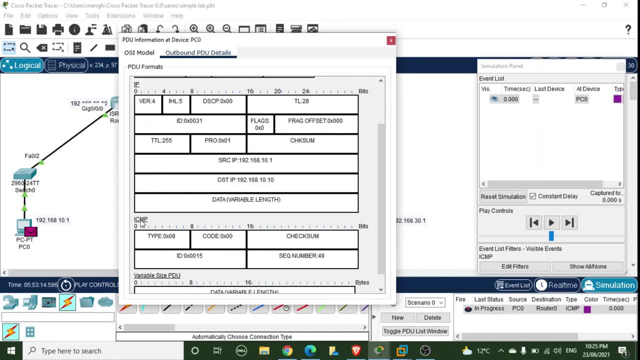 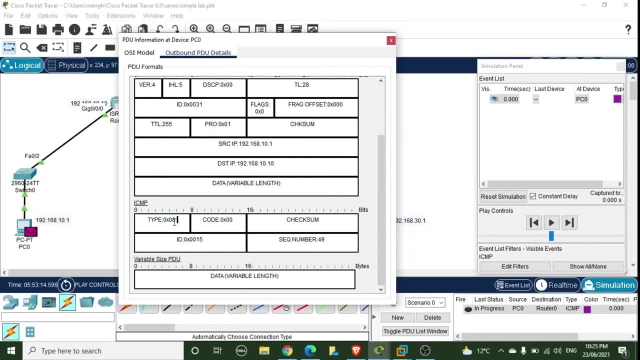 and within that ethernet we have this ip and then we have this icmp header and you can see, at the moment this type field is 0, 8, which is actually icmp type of messages, which is basically echo request message, and the code field we have 0. 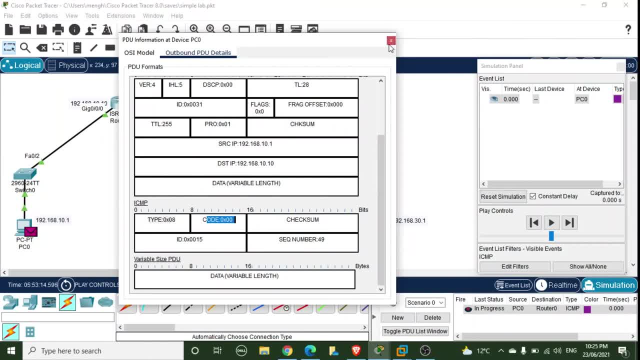 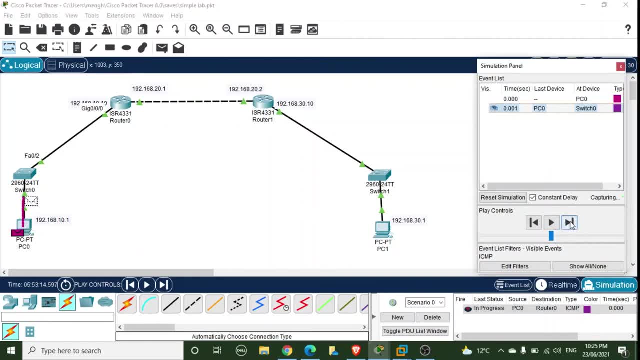 okay, so echo request type of message is being generated by this host or this source node and then this message goes to the switch and then switch forwards this message to the router and the router is actually reachable. so the router will send back a message that is known as echo reply and then this message is delivered to the actual source. 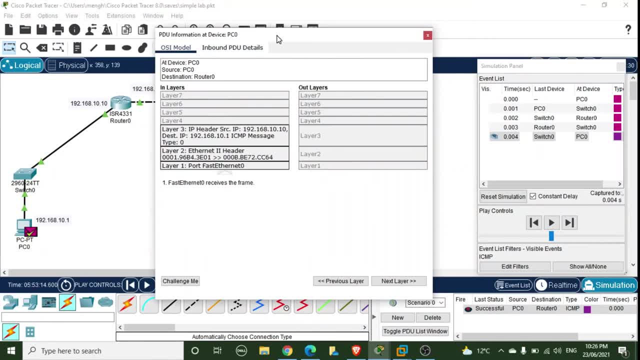 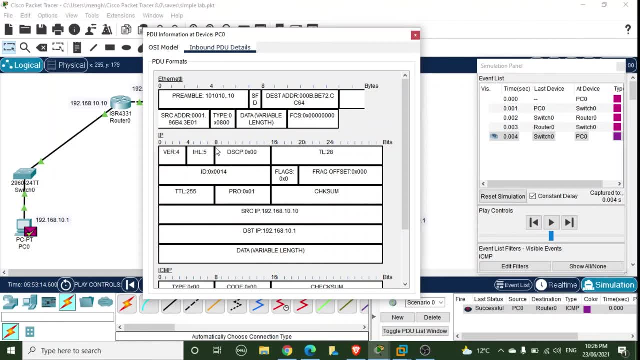 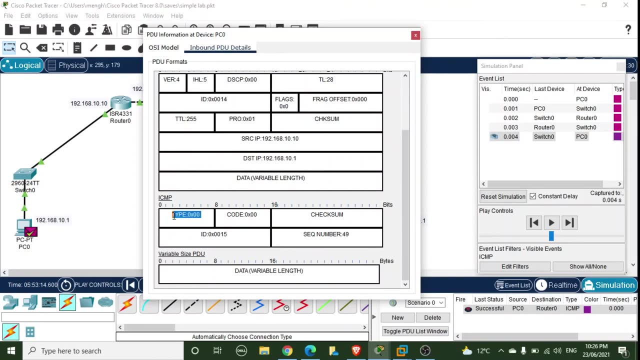 and now we want to see what is there after we have received back a message that is actually echo reply. so i'm going to click on this inbound pdu and this inbound pdu. if i scroll down, you can see this time the type: our icmp, a message type, is indicated by this code, that is 0: 0. 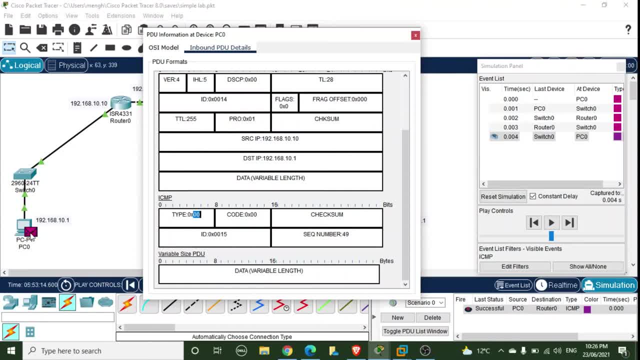 so that zero type indicates that this icmp message is basically echo reply message. so in this case this is all icmp messages which we discussed and you can switch the other, providing the code is that there is no compute error. so can further see on the wikipedia that we can have different icmp messages and those all icmp.